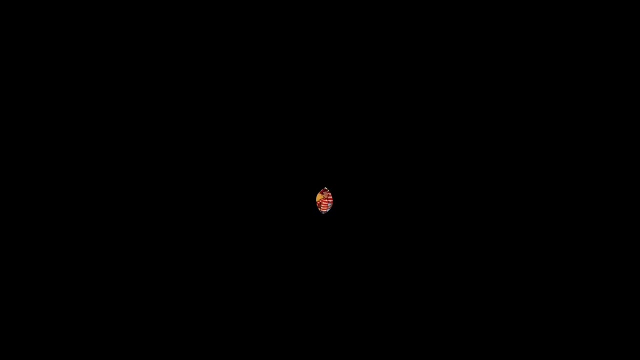 hand, you only see Waldo, but not Waldo's relative position in the image. Let's do another example with Watson on the left and Sherlock on the right. Sherlock has two spheres, one blue and one red. On the other hand, Watson is colorblind. 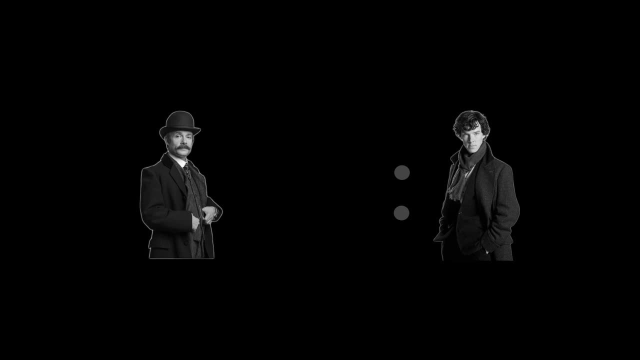 For Watson, both spheres look the same. Can Sherlock prove to Watson that he is not colorblind and can differentiate between the two spheres? Zero-knowledge requires that Sherlock does not reveal to Watson which sphere is blue and which sphere is red. Please take a moment to come up. 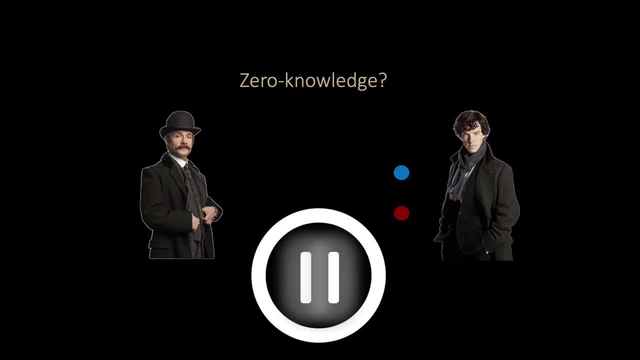 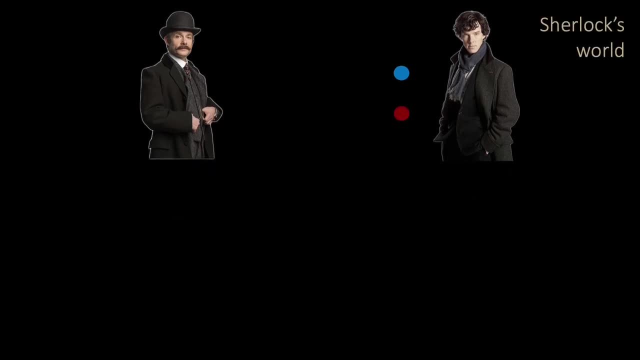 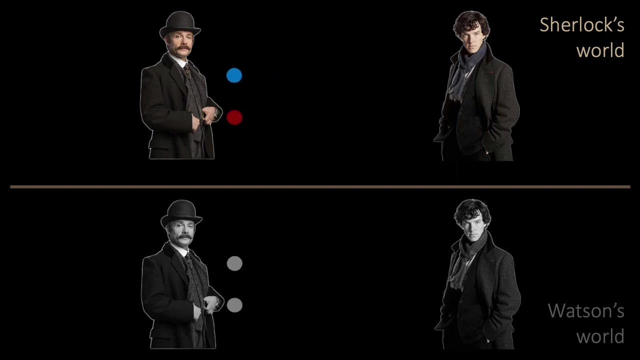 with a prover for this. Let's do another example, with Watson on the left and Sherlock on the right. Let us show how Sherlock and Watson experience the scene side by side. On top we have Sherlock's view. on the bottom is Watson's colorblind view. The protocol goes as follows: Watson takes the. 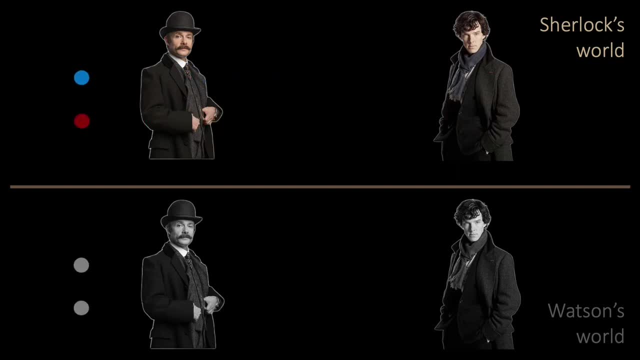 two spheres behind his back and he can choose to do one of the following: Keep the spheres as they are Or switch them. Next, Watson shows the spheres to Sherlock. Sherlock must tell whether Watson switched the spheres In this particular case. Sherlock must answer: switched, Of course. 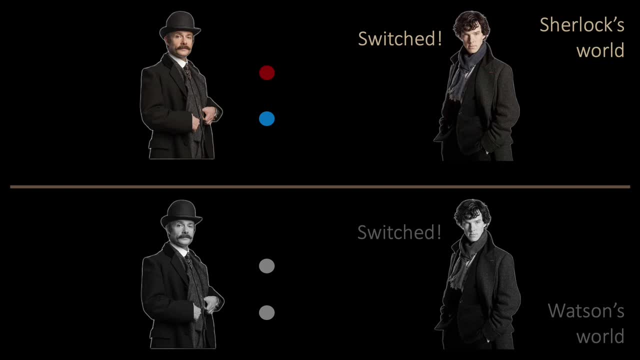 Sherlock might be lucky. so they repeat the protocol many times. If Sherlock always answers correctly, then Sherlock can distinguish the colors with a high probability, And none of Sherlock's answers reveal the color of the spheres. But we need to be careful. zero-knowledge is a 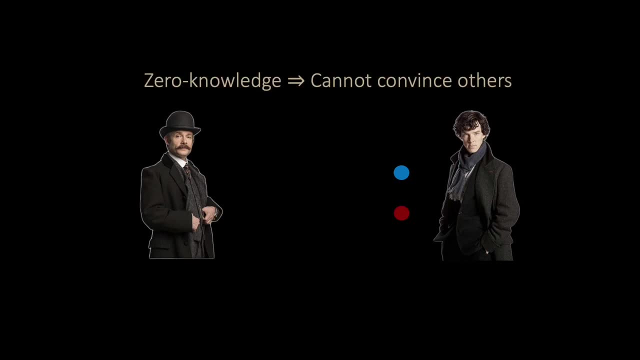 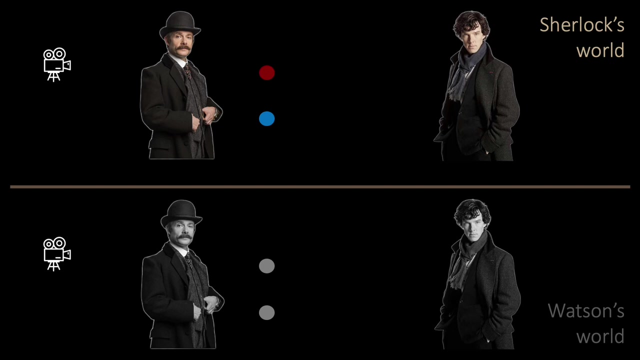 strong attribute. In particular, zero-knowledge demands that Watson cannot convince a third party that Sherlock can see the spheres. In this particular case, Sherlock must answer switched. Does our protocol fulfill this requirement? Say, Watson records the whole interaction with Sherlock as a movie and shows the recording to you. Will you be convinced that Sherlock can see? 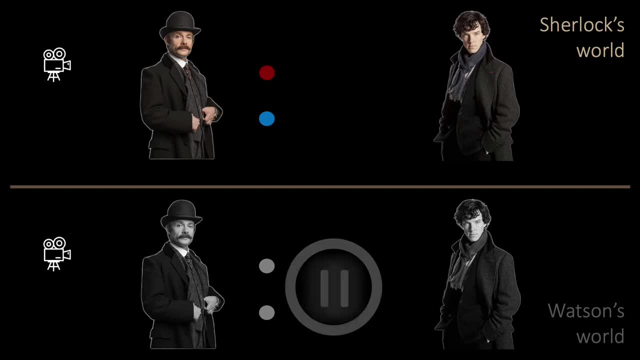 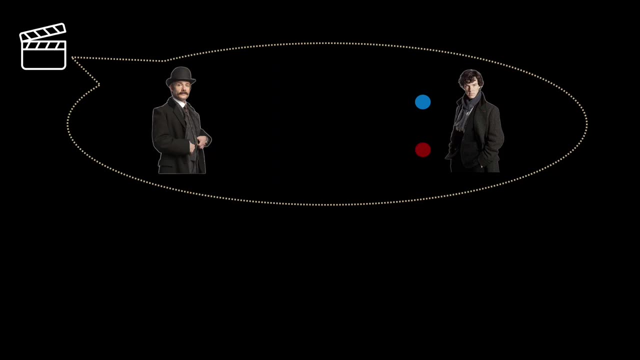 color. Pause the video to think about it. The movie cannot convince you that Sherlock can distinguish the colors, because Watson and Sherlock can create the same movie, even if Sherlock is colorblind. How can they do that? Sherlock and Watson can first decide in what? 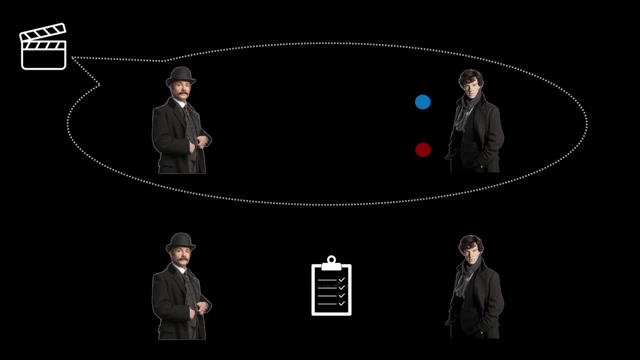 order to switch the spheres. In this particular case, Sherlock can distinguish the colors because Watson can distinguish the spheres. After they have agreed on the order, they start recording the movie. You can never tell whether it was a genuine recording where Sherlock was proving to Watson. 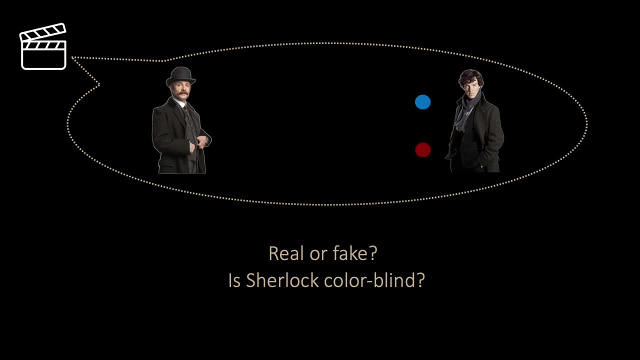 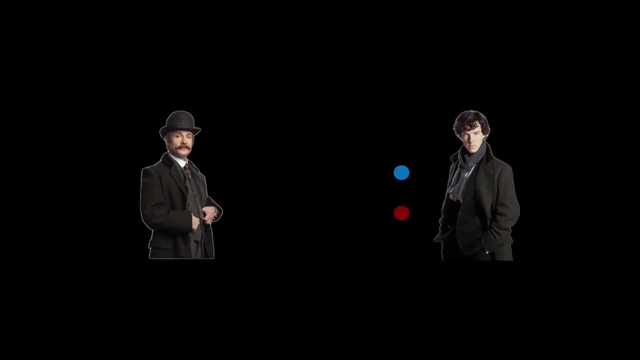 that he could distinguish the colors or whether they agreed on the order beforehand. So our protocol also fulfills this strong requirement. However, zero-knowledge needs an even stronger requirement. Zero-knowledge requires that Watson learns absolutely nothing, except that Sherlock can. 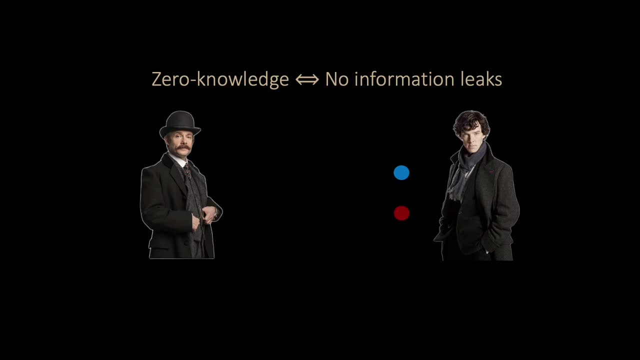 distinguish the colors. This must apply even if Watson is colorblind. If Sherlock is colorblind, Watson behaves dishonestly. Is there some way for Watson to trick Sherlock into revealing the colors of the spheres? Pause the video to think about it. Let us consider the case where Watson owns two. 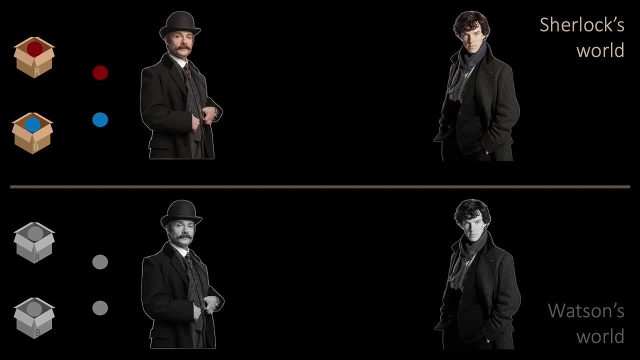 other spheres that look exactly like Sherlock's. In addition, let us assume that Watson's spheres are secretly marked, so Watson knows which one is red and which one is blue. Now he can do the following trick: First, Watson shows Sherlock's spheres. 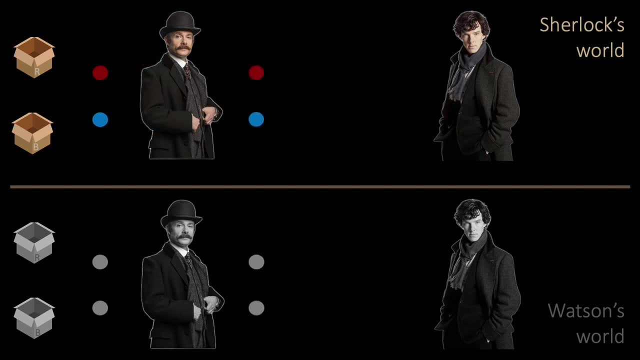 But then Watson shows his marked spheres. Based on Sherlock's answer, Watson can now infer the colors of Sherlock's spheres. For example, if Sherlock answers not switched, Watson can map the colors as shown here At the beginning of the protocol. Watson only knew the colors of his. 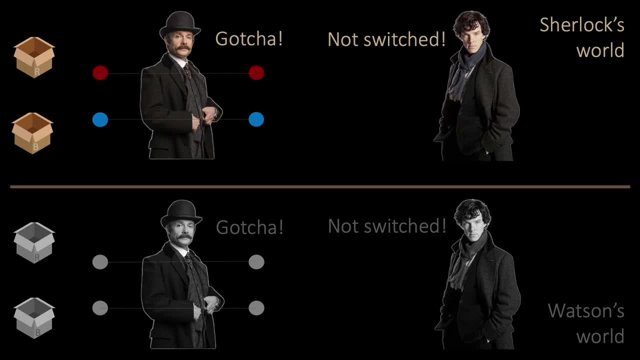 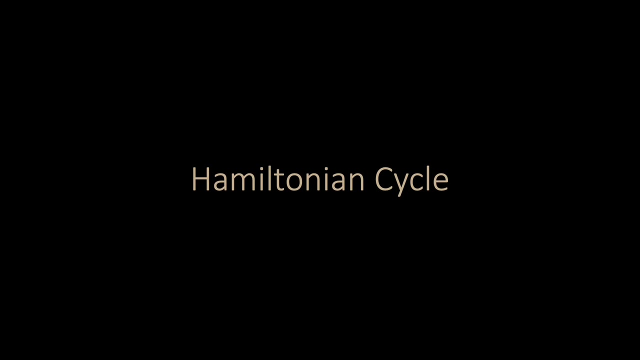 spheres, But now Watson knows the colors of all four spheres. Thanks to the protocol, Watson learned the colors of Sherlock's spheres. Hence the protocol is not zero-knowledge. Another example of a zero-knowledge proof is the Hamiltonian cycle problem. Hamiltonian cycle is 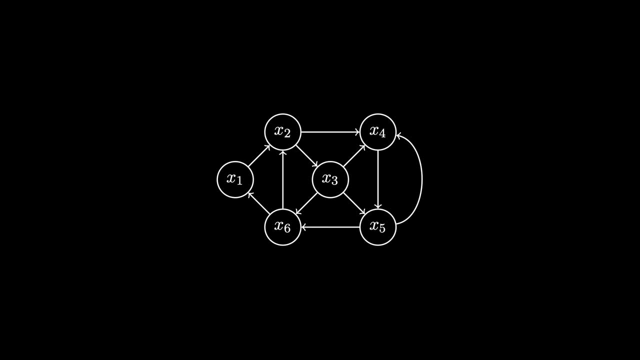 the problem of finding a cycle in a graph that visits each node exactly once. A possible solution is shown here. Of course, in this small example it is easy to find such a Hamiltonian cycle, but in general Hamiltonian cycle is a known NP-hard problem. This means that a zero-knowledge 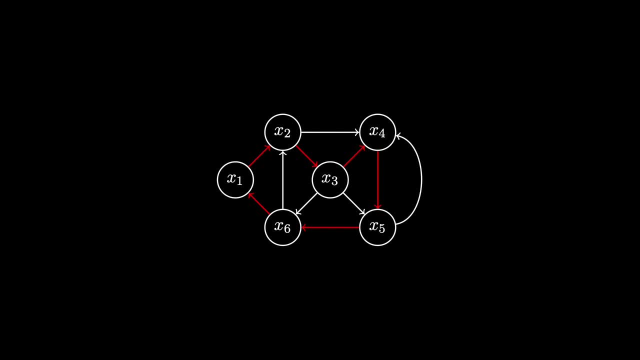 proof for Hamiltonian cycle can be used as a zero-knowledge proof for every problem. in NP We can represent a graph with an adjacency matrix. So let's assume that Sherlock knows a Hamiltonian cycle in the graph and Watson does not. Sherlock wants to prove to Watson that he. 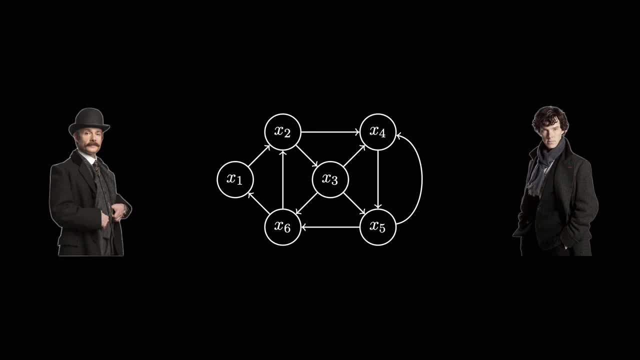 knows the cycle without revealing anything else. How can Sherlock do that? Take a moment to think about potential protocols. First Sherlock tells Watson to look away. Then Sherlock creates a permutation of the graph by simply permuting the names of each node. Then Sherlock creates a. 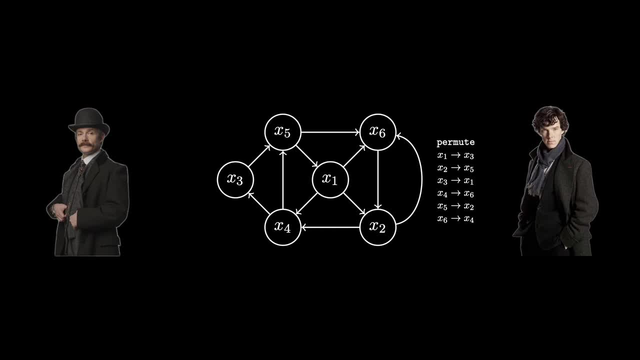 permutation of each node in the graph. For example, Sherlock renames x1 with x3, x2 with x5, and so on. This leads to permuted adjacency matrix. Sherlock only uses the adjacency matrix, hides every entry of the permuted matrix and tells Watson to look back. Watson now has two choices. 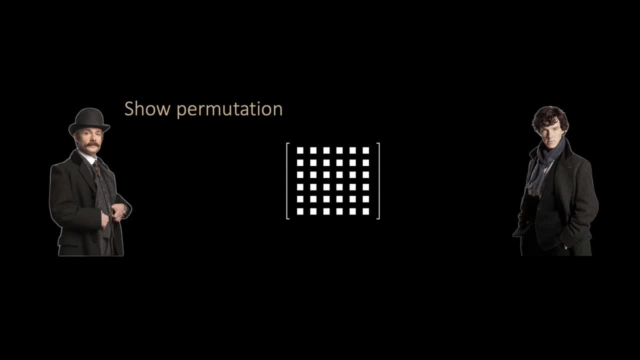 He can request Sherlock to open the matrix and show the permutation. Sherlock can do this by opening every matrix entry and showing how he changed the names. Watson's second option is to ask for the cycle. In this case, Sherlock only shows the entries that 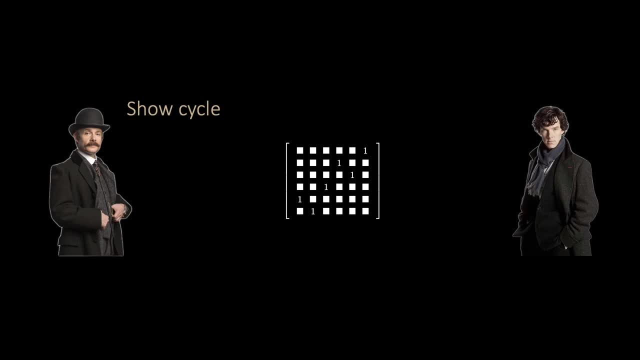 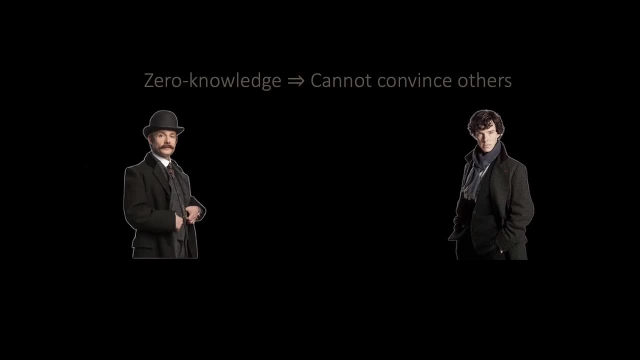 make up a cycle. They repeat the protocol many times and in each repetition Watson can either ask for the permutation or for the cycle, but never for both. Can Watson convince a third party that Sherlock knows the cycle? Take a moment to think about it, Even if Sherlock does not know. 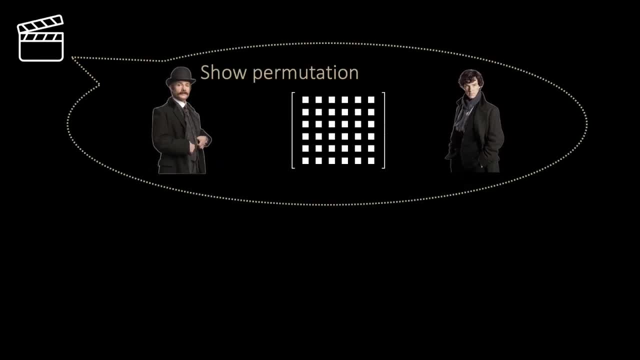 the cycle. Watson and Sherlock can create the same movie by agreeing on the order of the cycle. If the challenge is to open the permutation, Sherlock hides a random permutation of the graph. This way he can easily answer show permutation challenge. If the challenge is to open a cycle, 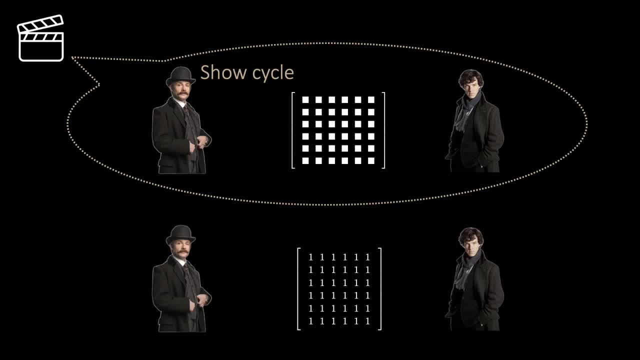 Sherlock hides a matrix that contains only ones. This way, Sherlock can also easily open a random cycle. Note that Sherlock knows the challenge before each round, since Watson and Sherlock agreed on the order. Similar to the colorblind example, you can never tell what the order is. 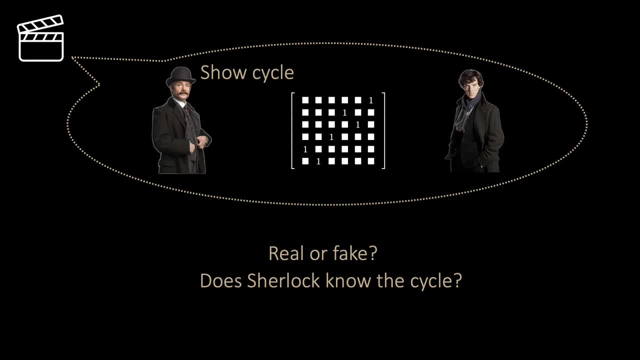 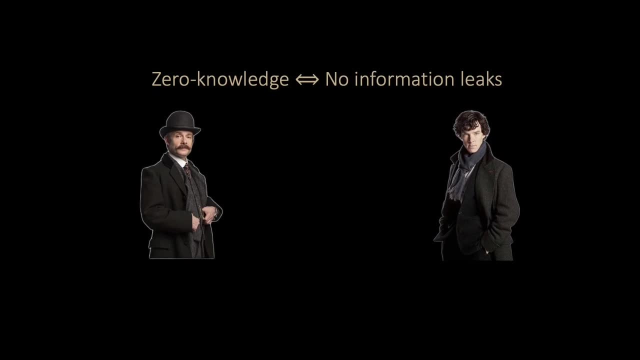 Whether it is a genuine recording or the one where Watson and Sherlock decided on the order beforehand. However, as mentioned before, zero knowledge is a stronger property and states that no information leaks. One can show that Hamiltonian cycle is zero knowledge, However, to do so, 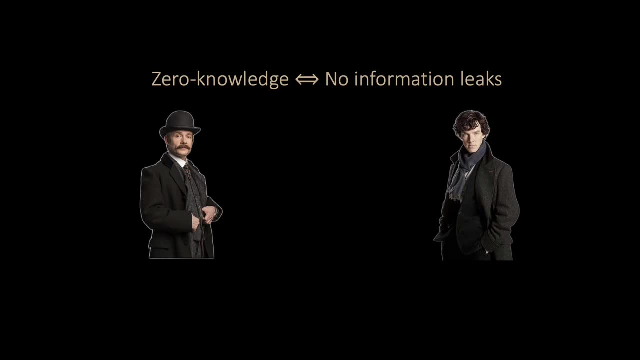 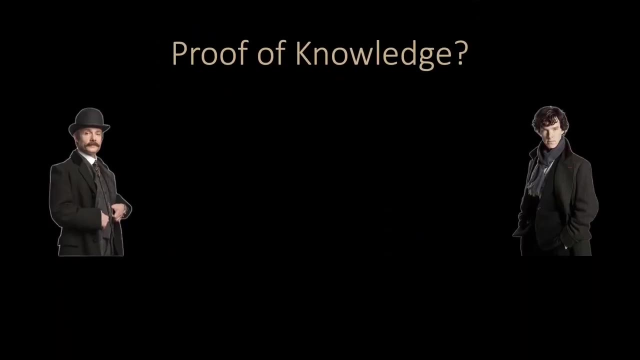 we need a more formal model. Such a formal model exists, but we cannot explain the details in this video. But why should Watson be convinced that Sherlock knows the cycle? If Sherlock can answer questions, he knows a Hamiltonian cycle in the graph, since he can simply revert the permutation. 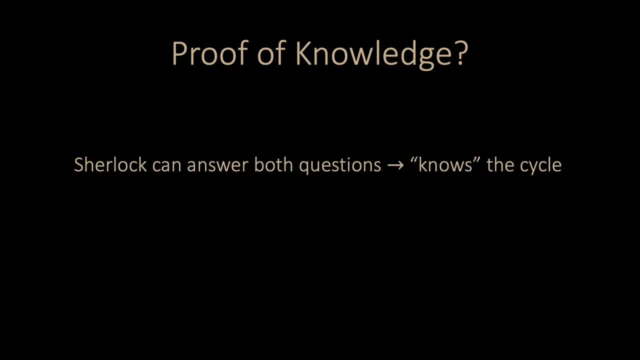 and get the cycle in the original graph. So if Sherlock can answer both questions, it follows that Sherlock knows the cycle. Conversely, if Sherlock does not know the cycle, he can answer only one question. If Sherlock does not know the cycle.